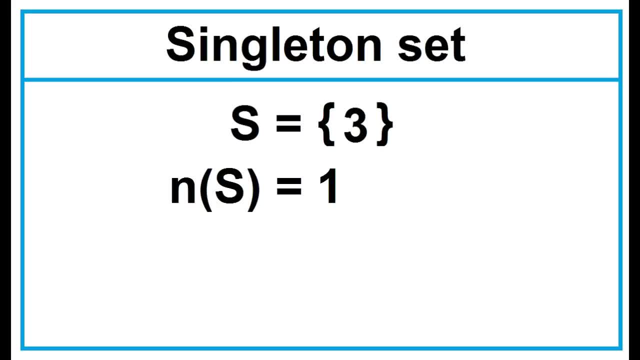 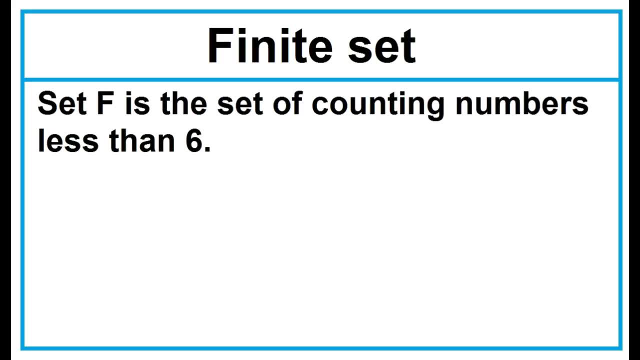 singleton set. The cardinality of set S is one Finite set A set with limited elements. Example: Set F is the set of counting numbers Less than six. The elements of set F are one, two, three, four, five. The cardinality. 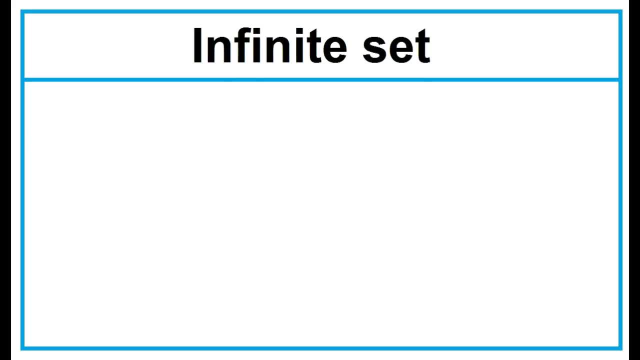 of set F is five Infinite set, A set with unlimited elements. Example: Set N is the set of counting numbers. The elements of set N are one, two, three and so on. The cardinality of set N is infinite. 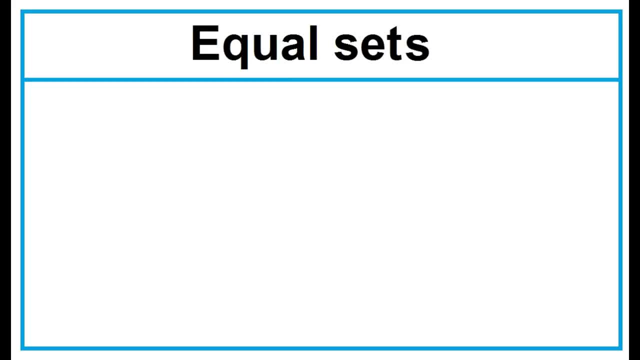 Equal sets. Two sets are equal if they have the same elements. Example: Set E is the set of letters in the word Earth. The elements of set E are E, A, R, T H. Set H is the set of letters in the word heart. The elements of set H are E, A, R T H. 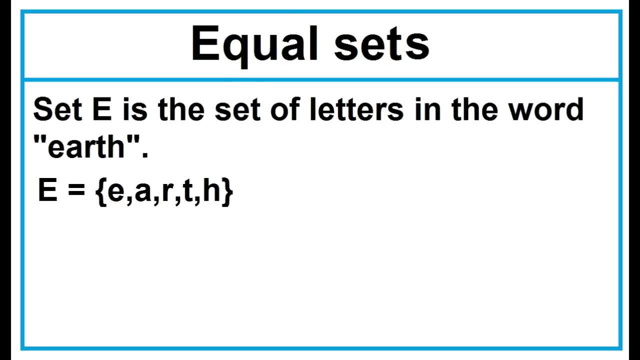 Set L is the set of letters in the word heart, The elements of set L». Or we can say set H, Test E. Or you can say strawberry reached high. Or you can say blueberry reached. Or you can say strawberry reached. That's it. Then let's talk about numbers, and that is the same for cardinality of set E. The term Segis can also be used: Ca circa لا. The servic sacrifice can also be taken into credit For a problem students may have anized oribilical analysis. 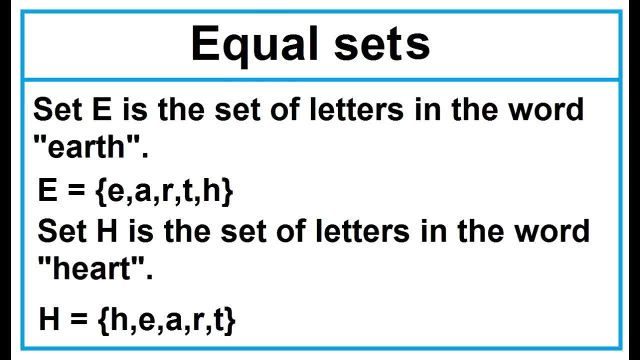 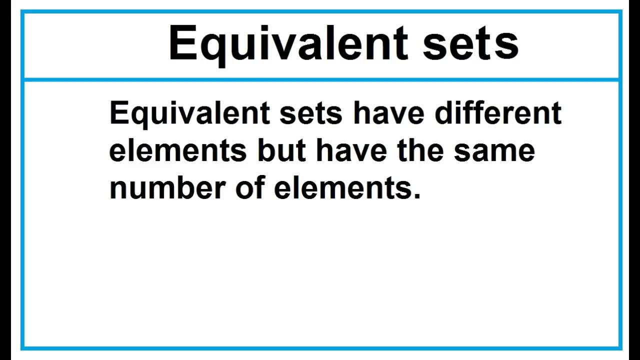 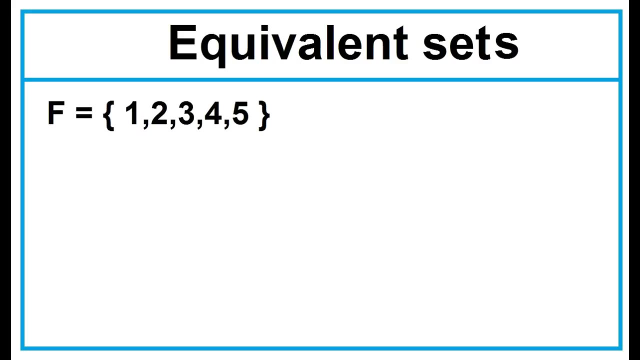 are t. Set E and set H have the same elements. They are equal sets. Set E equals set H, Equivalent sets. Equivalent sets have different elements but have the same number of elements. Example given: set F and set H. The cardinality of set F is five and the cardinality of set H is 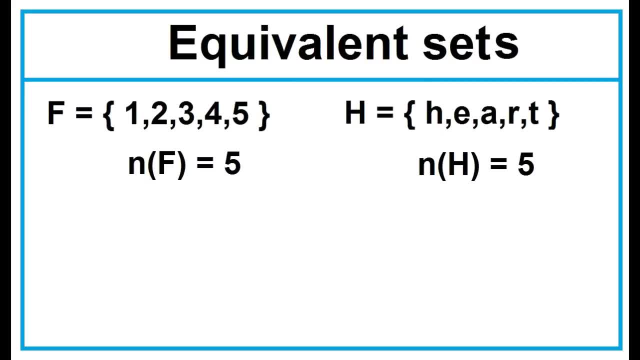 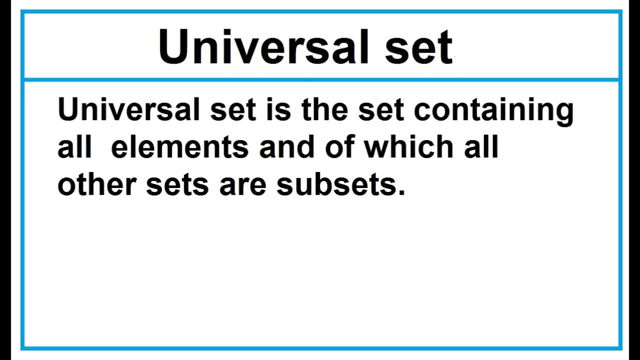 five. The two sets have different elements, but they have the same number of elements. Set F is equivalent to set H, Universal set. Universal set is the set containing all elements and set H And of which all other sets are subsets. The universal set is represented by a capital letter. 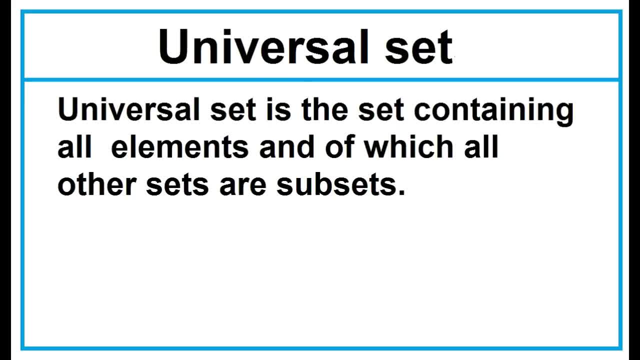 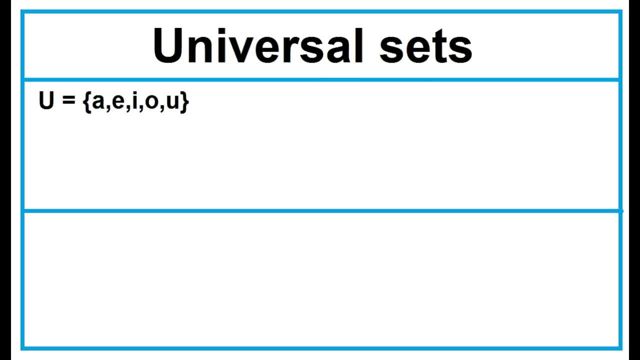 U Example, let U be the universal set. Set U is the set of all vowels in the English alphabet. All other sets are subsets of the universal set. Set A is a proper subset of set U. Set B is also a proper subset of set U. 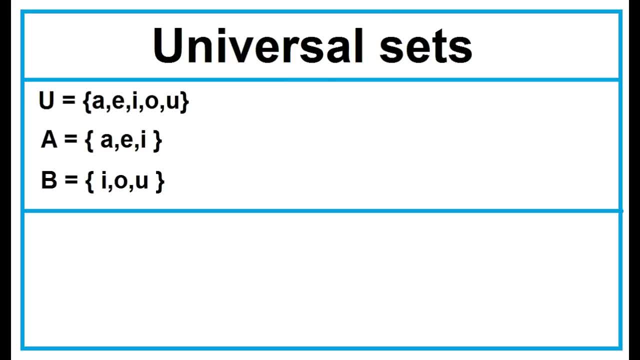 All the elements of sets A and B are also found in the universal set. Another example: Set U is the set of counting numbers. Sets A, B and C are proper subsets of set U, because a universal set contains all the elements in a particular problem Subset. 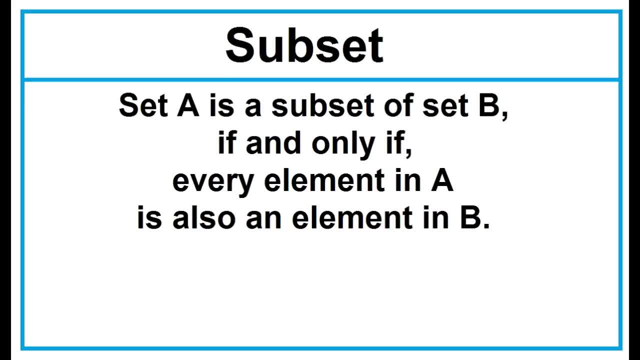 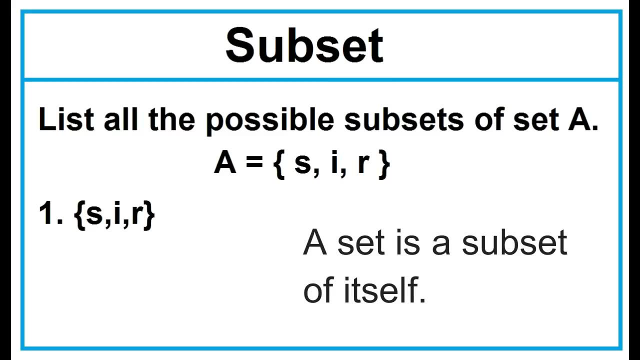 Set A is a subset of set B if, and only if, every element in A is also an element in B. Here's an example List all the possible subsets of set A: 1. A set with 3 elements: 2,, 3, 4. 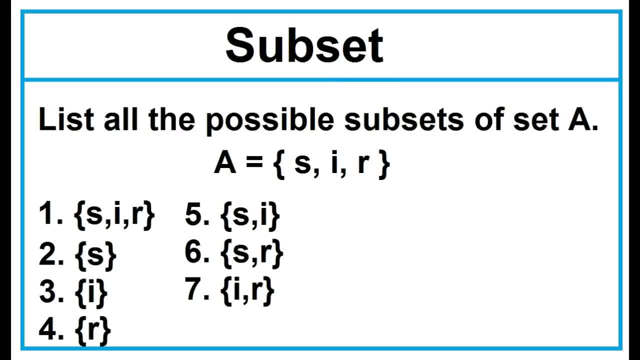 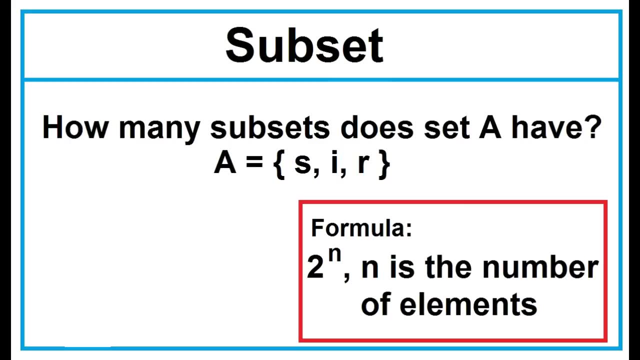 2,, 3,, 4, 2, 3, 4 Sets with 1 element, 5,, 6,, 7 Sets with 2 elements And number 8 is an empty set. How many subsets does set A have? To find the number of subsets, use this formula. 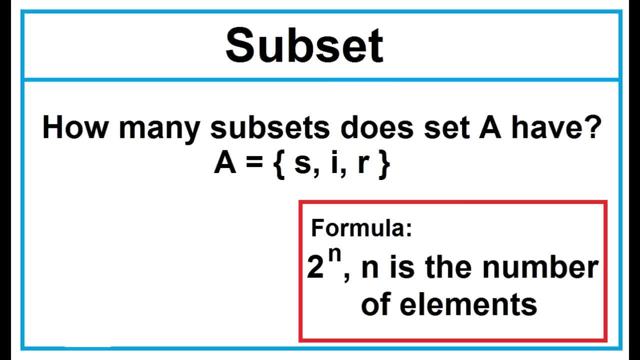 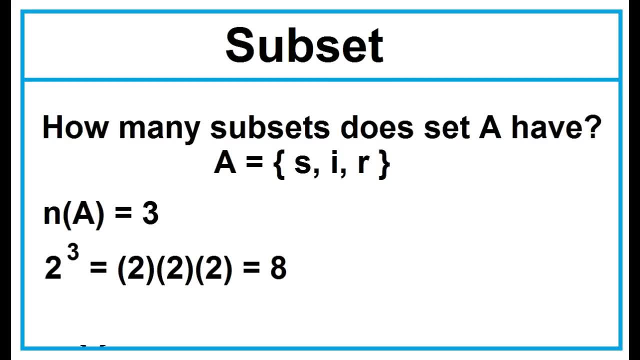 2 to the power of n, where n is the number of elements. The cardinality of set A is 3, So 2 to the power of n. 2 to the power of 3 is just 2 times 2 times 2 equals 8. 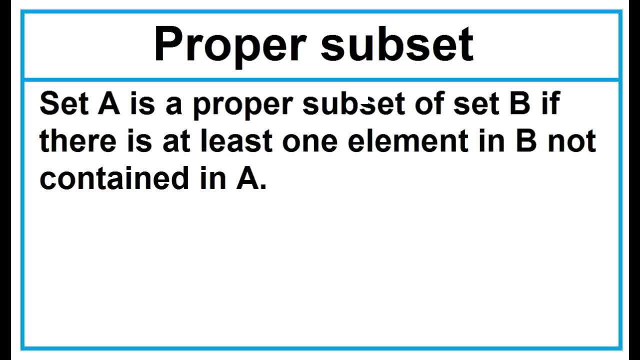 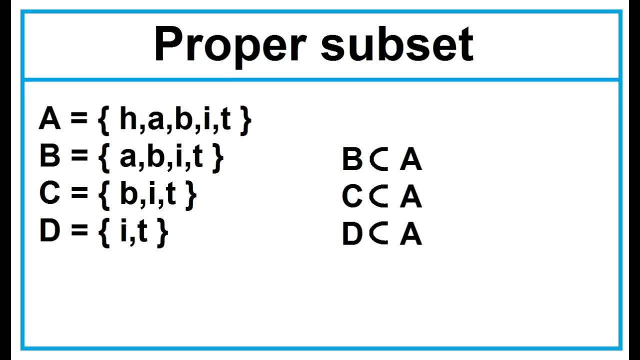 Proper subset. Set A is a proper subset of set B if there is at least one element in B not contained in A In symbol, Set A is a proper subset of set B. Example Given: Sets A, B, C and Z are proper subsets of set B. 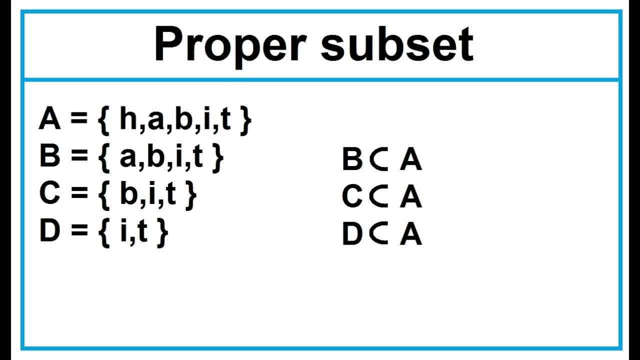 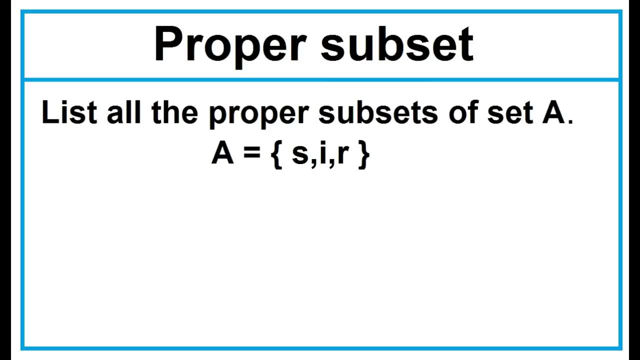 Set B is a proper subset of set A. Set C is a proper subset of set A. Set D is a proper subset of set A. List all the proper subsets of set A. Sets 1,, 2, 3 have 2 elements. Sets 4, 5, 6 have 1 element. 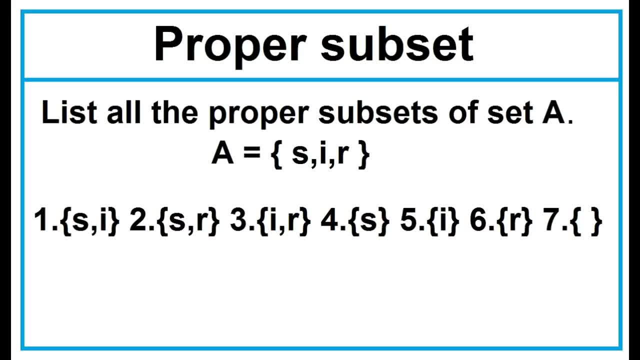 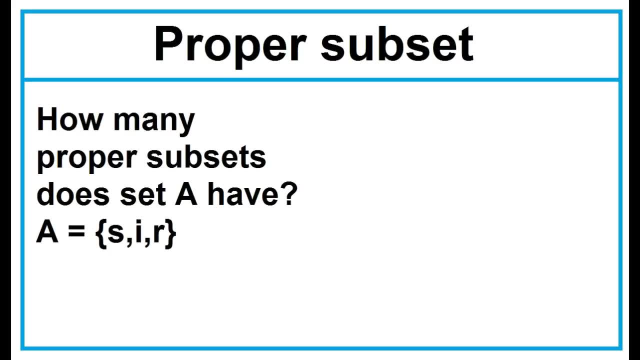 Sets 5, 6 have 1 element And number 7 is an empty set. The set itself is not a proper subset of set A. How many proper subsets does set A have, Since the set itself is not a proper subset? The formula is 2 to the power of n. 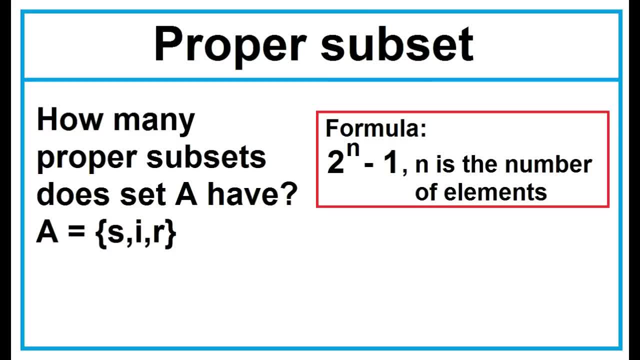 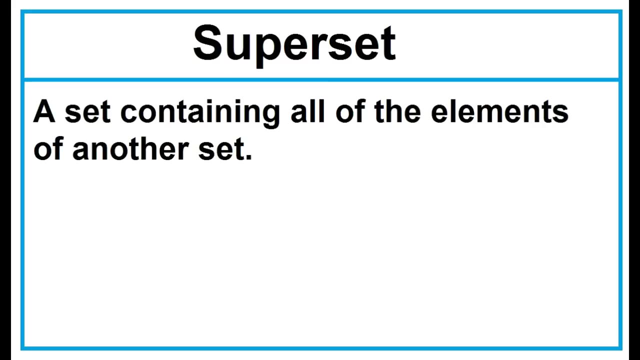 minus 1, where n is the number of elements. The cardinality of set A is 3.. Using the formula 2 to the power of 3 minus 1 equals 8 minus 1 is 7.. Supperset: Supperset is a set containing all of the elements of another set. 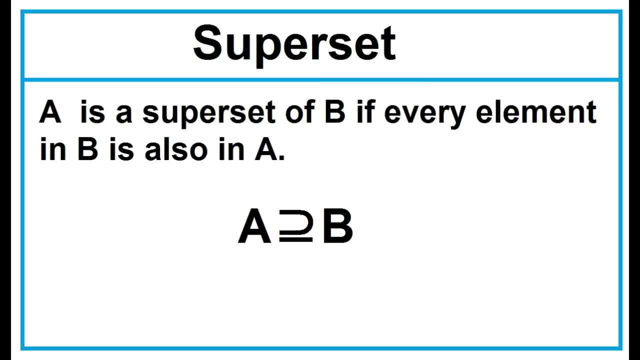 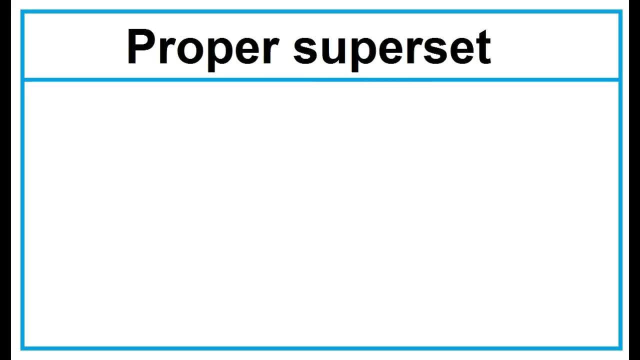 Symbol: set A is a superset of set B. This is just a reverse of subset Proper supperset. Set A is a proper supperset of set B if set A is a supperset of set B and set A is not equal to set B. 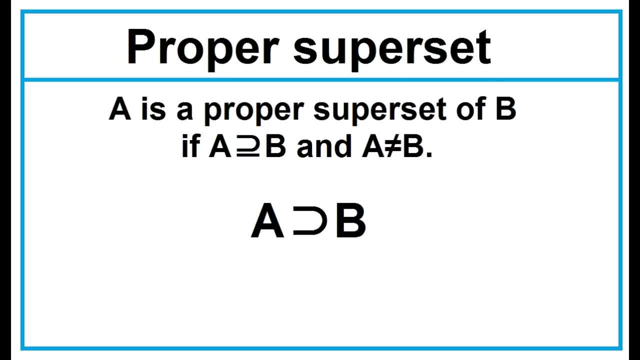 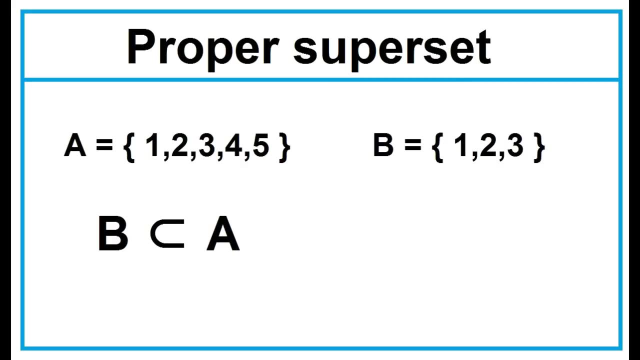 In symbol. set A is a proper supperset of set B. Given set A and set B, While set B is a proper subset subset of set A. set A is a proper supperset of set B. Power set: The set of all the subsets of a set. 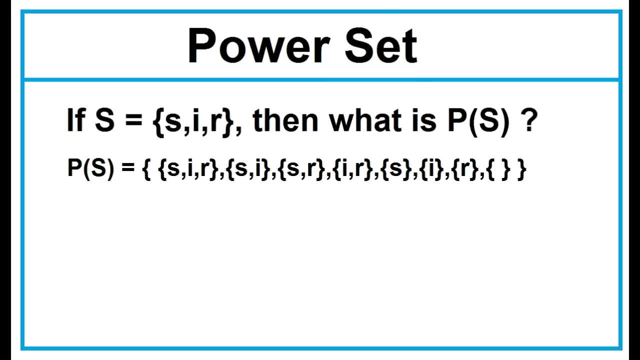 What is the power set of set S? P of S contains all the subsets of set S. How many elements does the power set of set S have? Since a power set contains all the subsets of a given set, it follows the formula 2 to the power of n.